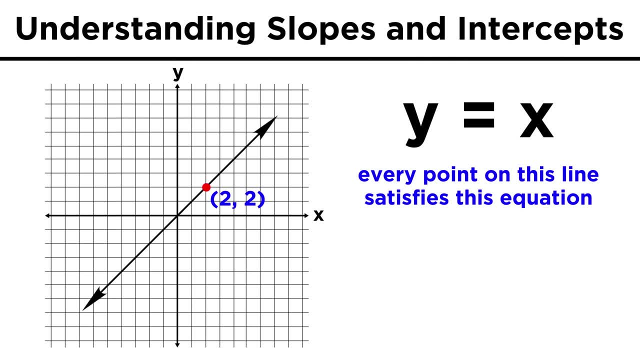 to plot this line. so here it is, with every point showing an ordered pair where the X and Y values are equivalent To calculate the slope. we must understand that this is equal to rise over run, which means change in Y over change in X. 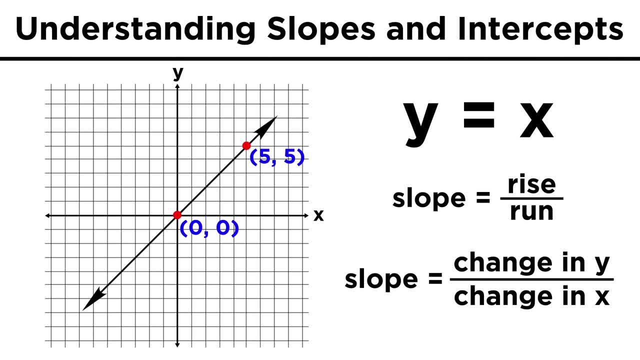 We can pick any two points on this line and with these points we take the difference in their Y values and divide by the difference in their X values. Y is up and down or the rise, and X is side to side or the run. 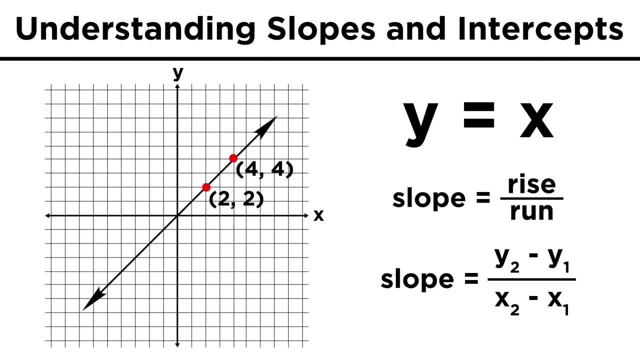 Rise over run. Let's pick these two points: two, two and four. four Rise over run can be represented this way: Y two minus Y one, Y two minus Y one over X, two minus X one. so we just plug the coordinates in. 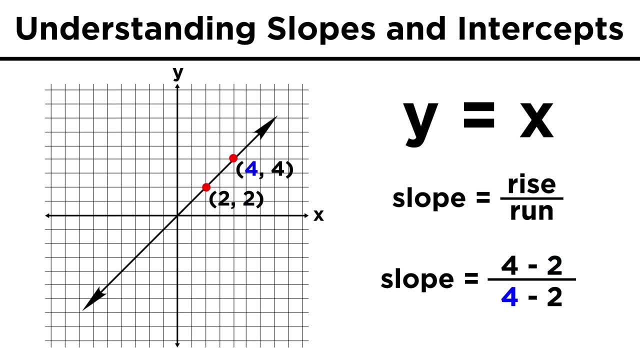 Y two is four, Y one is two, X two is four and X one is two. We simplify and get two over two or one. The slope of this line is one That should make sense, because Y equals X is in, Y equals MX plus B form. it's just. 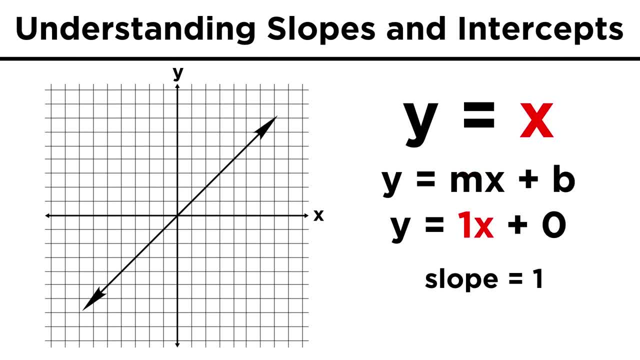 that M is one and B is zero. One X is just X and B is zero because the line crosses the Y axis when Y equals zero. so we get this very simple equation: Y equals X. If a line has a slope that is greater than one, it will tilt upwards like this steeper. 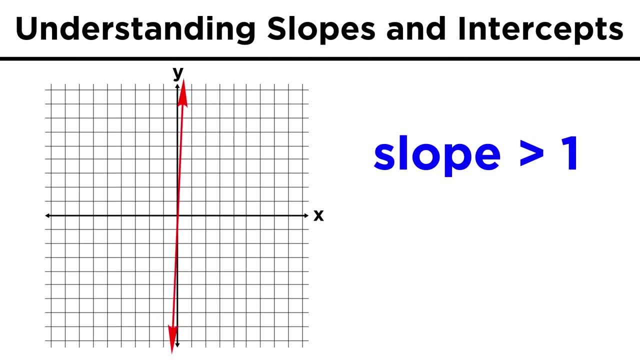 and steeper climbing towards infinity, until it reaches complete verticality, at which point the slope is undefined, Because the line rises all the way to infinity in the Y direction without any run at all, and infinity over zero is undefined. If, instead, the slope is less than one, the line tilts downwards, this way, the slope getting 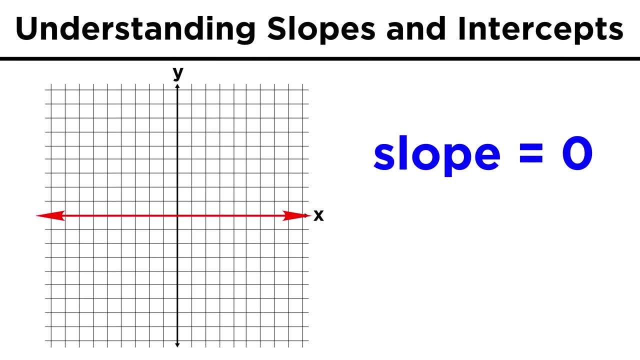 smaller and smaller until it is completely horizontal, at which point the slope will become zero. The line runs all the way to infinity in the X direction without rising at all, and zero over infinity is zero. So vertical lines have an undefined slope, horizontal lines have zero slope and everything. 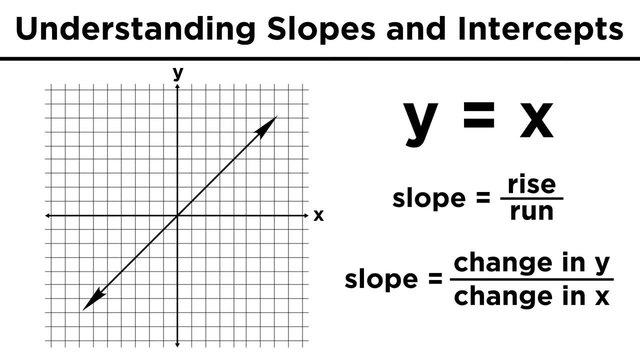 values are equivalent To calculate the slope. we must understand that this is equal to rise over run, which means change in Y over change in X. We can pick any two points on this line and with these points we take the difference in their Y values and divide by the difference in their X values. 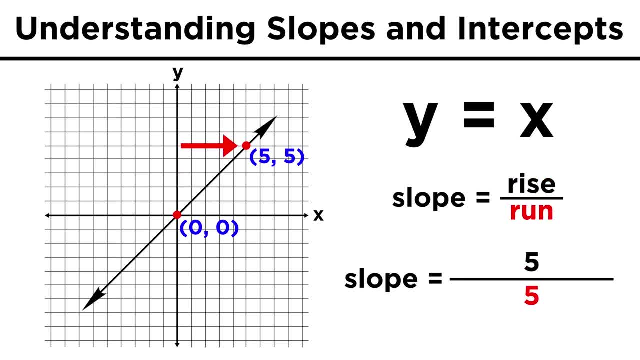 Y is up and down or the rise, and X is side to side or the run, Rise over run. Let's pick these two points: two, two and four. four Rise over run can be represented this way: Y two minus Y one over X, two minus X one. 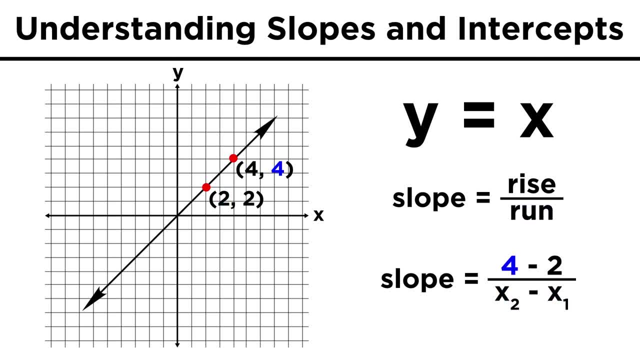 so we just plug the coordinates in: Y two is four, Y one is two, X two is four and X one is two. We simplify and get two over two or one. The slope of this line is one That should make sense. 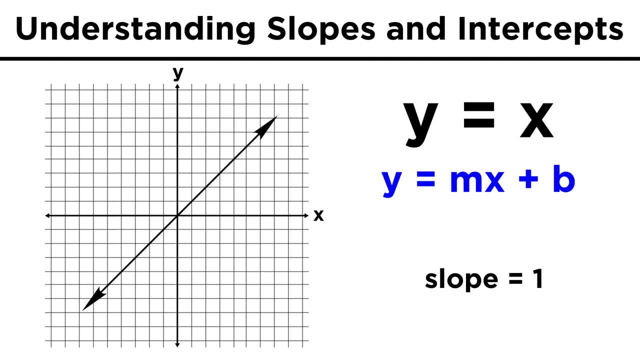 Because Y equals X is in Y equals M, X plus B form. It's just that M is one and B is zero. One X is just X and B is zero because the line crosses the Y axis when Y equals zero. so we get this very simple equation: Y equals X. 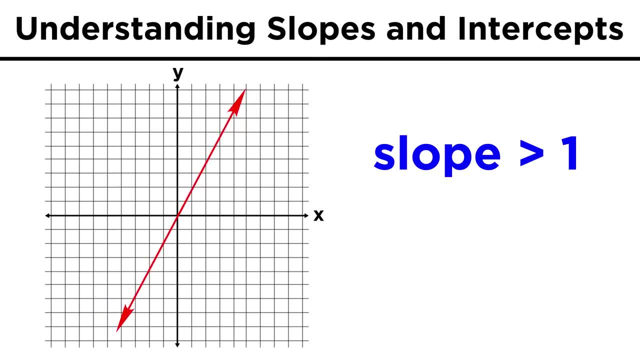 If a line has a slope that is greater than one, it will tilt upwards like this, steeper and steeper Towards infinity, until it reaches complete verticality, at which point the slope is undefined, because the line rises all the way to infinity in the Y direction without any run at all. 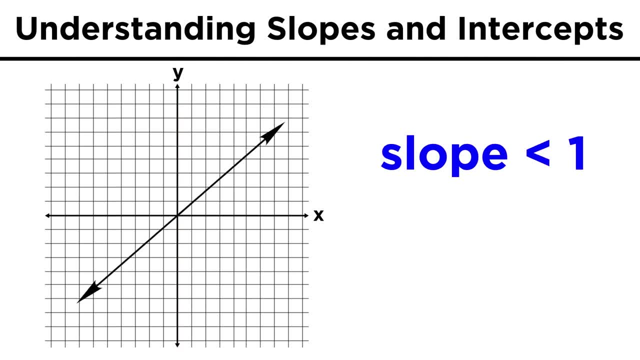 and infinity over zero is undefined. If, instead, the slope is less than one, the line tilts downwards. this way, the slope getting smaller and smaller until it is completely horizontal, at which point the slope will become zero. The line runs all the way to infinity in the X direction without rising at all, and zero. 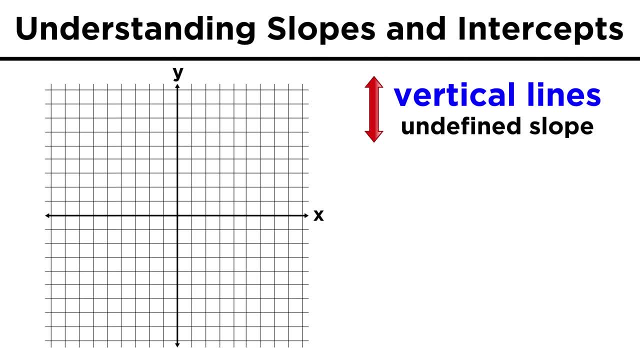 over infinity is zero. So vertical lines have an undefined slope, horizontal lines have zero slope and everything in between has some slope between zero and infinity. If we continue past the horizontal, the slope becomes increasingly negative because as we run in the positive direction, we're going to have a slope that is greater than 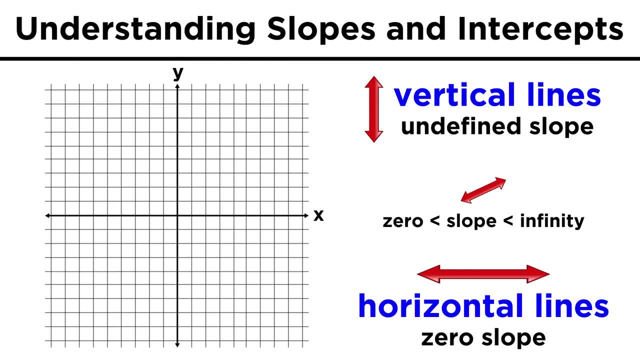 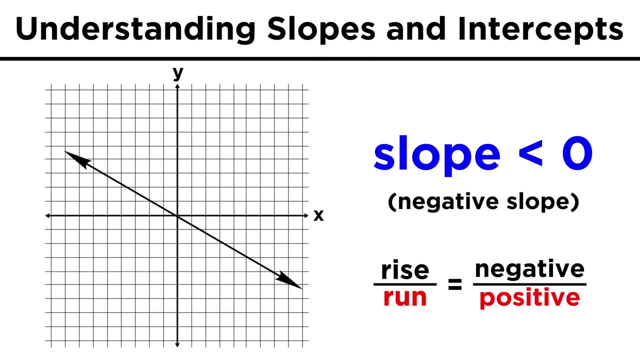 in between has some slope between zero and infinity. If we continue past the horizontal, the slope becomes increasingly negative because, as we run in the positive direction, the rise is negative or, moving downwards, The slope will increase in the negative direction, approaching negative. 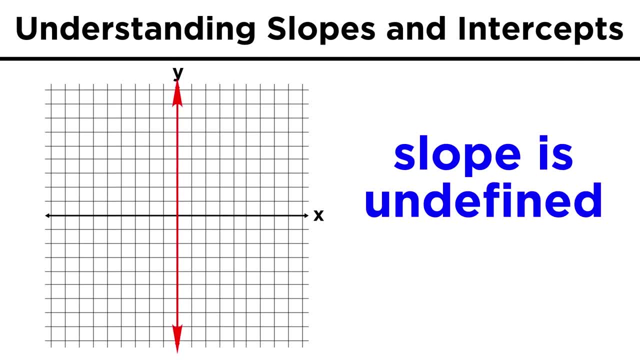 And if the slope is definitely undefined, then the slope towards infinity will rise to negative infinity until vertical, where the slope becomes undefined. Let's just quickly mention that any two points define a line. You could draw any two points at random on the coordinate plane and there is a line. 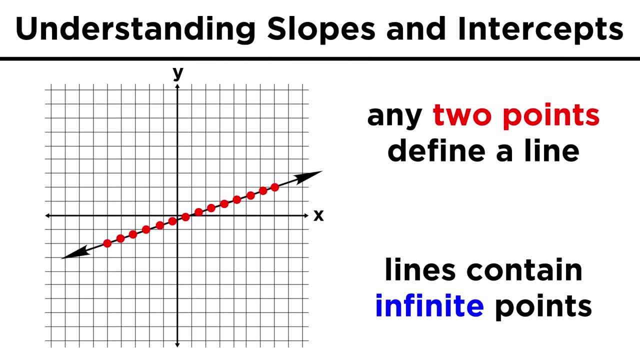 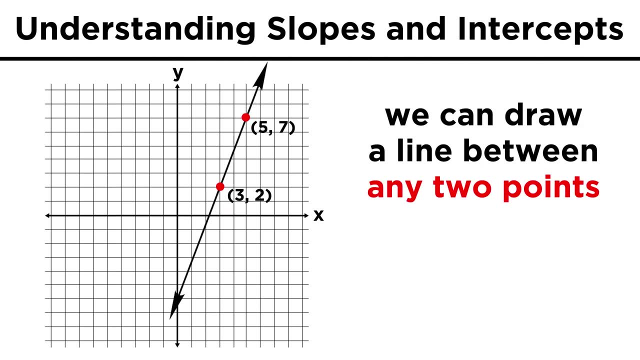 that connects them. However, all lines contain an infinite number of points, since the coordinates can become infinitely precise. an X and Y value that qualifies as a solution to the equation. We could pick two points like three, two and five, seven, and draw a line between them. 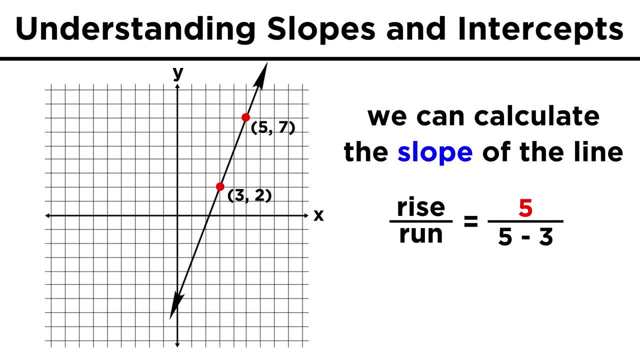 We could also calculate the slope: Seven minus two is five, and five minus three is two, so the slope is five halves. Always remember that when calculating slope, it doesn't matter which point is point one and which is point two, but the coordinates of each point must remain together. so, whichever, 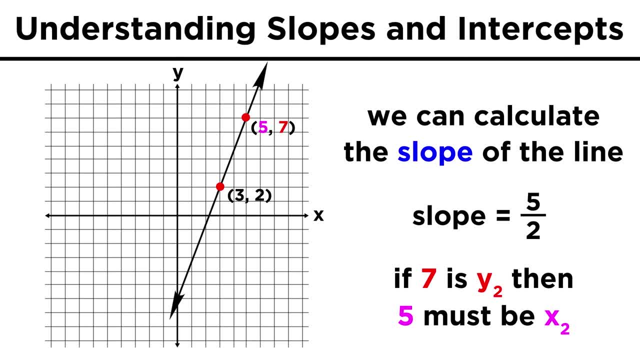 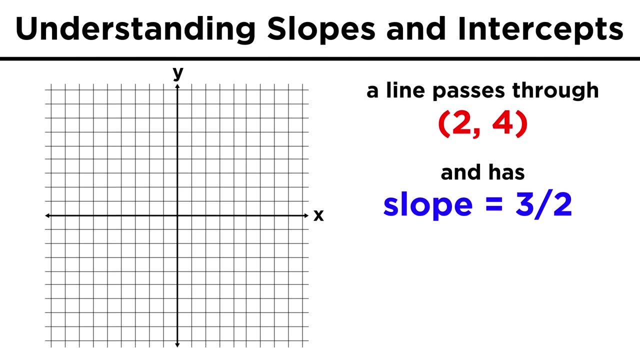 Y value is Y two. the X value in that point must be X two and not X one. That would lead to an incorrect slope calculation. Also, one point and a slope can define a line. We could say that a line passes through two, four and has a slope of three halves. 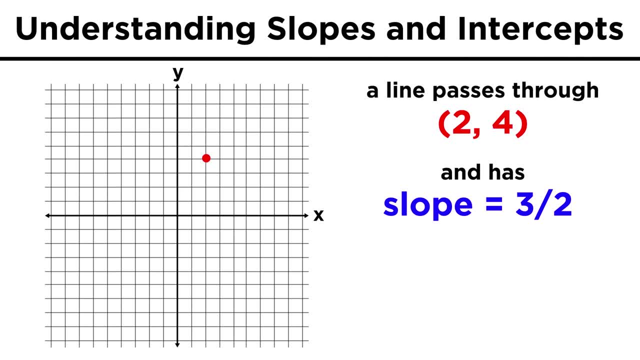 To draw this line, we would just go to the point two, four And start applying the slope Up three over two. This could also be down three, two to the left, because negative three over negative two also equals three halves, and that's how the slope which we can regard as the 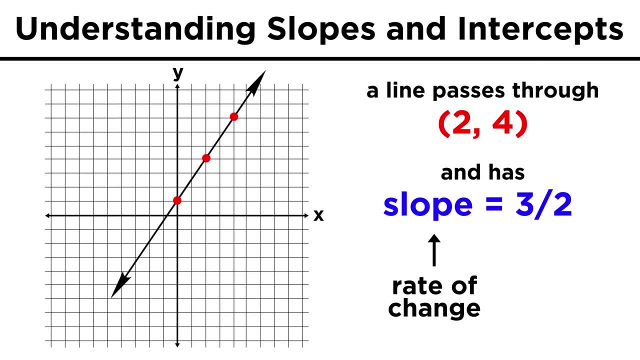 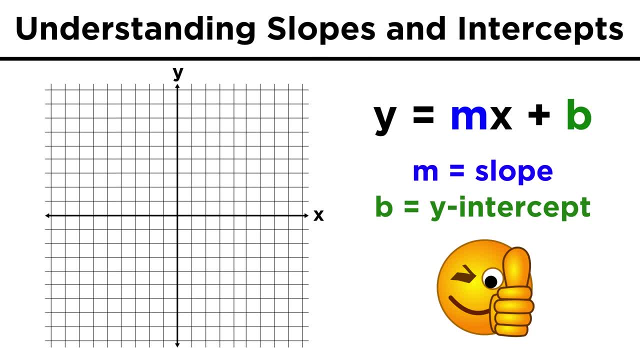 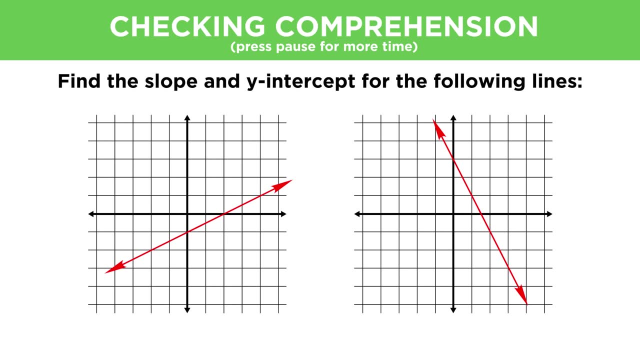 rate of change makes sense regardless of which direction you travel. Now that we understand slopes and Y intercepts, let's check comprehension. Thanks for watching, guys. Subscribe to our channel for more videos like this one. Subscribe to my channel for more tutorials. 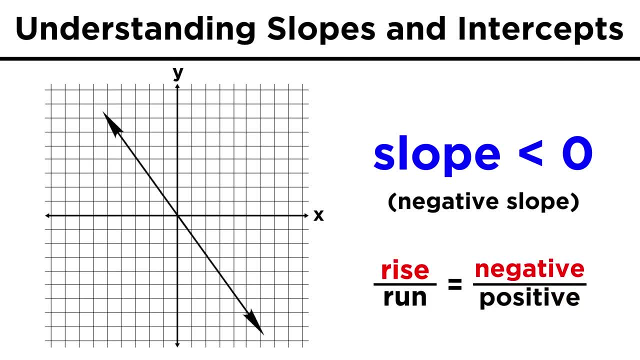 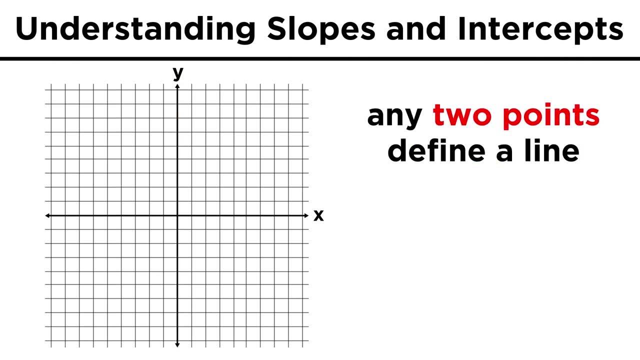 zero direction. the rise is negative or moving downwards. The slope will increase in the negative direction, approaching negative infinity, until vertical, where the slope becomes undefined. Let's just quickly mention that any two points define a line. You could draw any two points at random on the coordinate plane and there is a line. 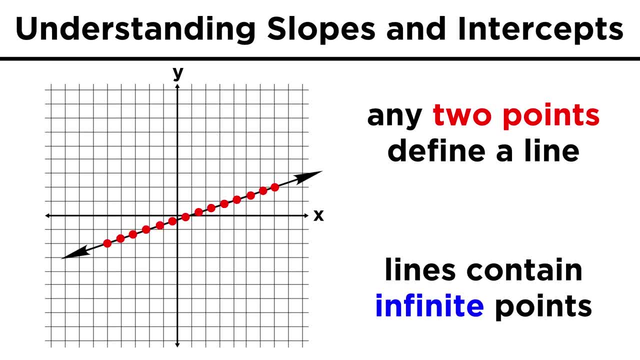 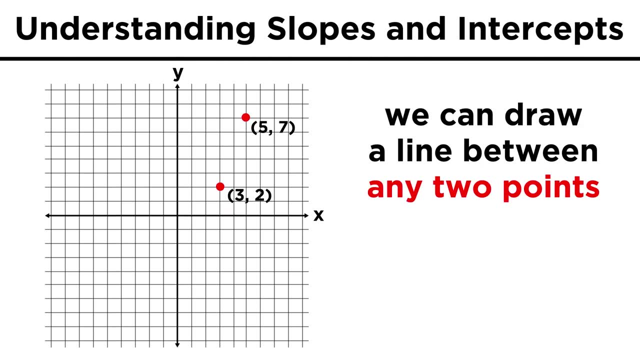 that connects them. However, all lines contain an infinite number of points, since the coordinates can become infinitely precise and any point on the line represents an X and Y value, that qualifies as a solution to the equation. We could pick two points like three, two and five, seven, and draw a line between them. 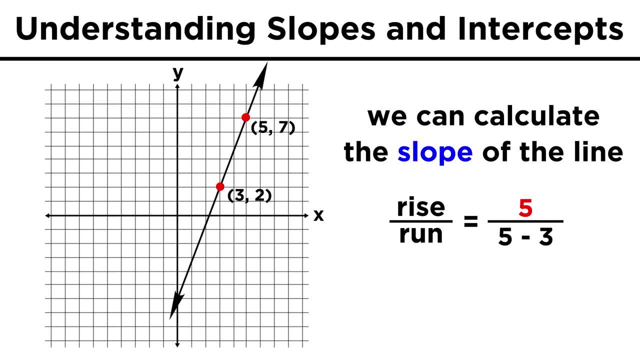 We could also calculate the slope: Seven minus two is five, and five minus three is two, so the slope is five halves. Always remember that when calculating slope, it doesn't matter which point is point one and which is point two, but the coordinates of each point must remain together. 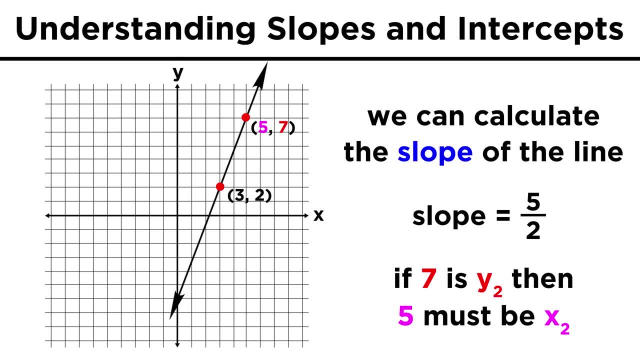 So whichever Y value is Y two, the X value in that point must be X two and not X one. That would lead to an incorrect slope calculation. Also, one point and a slope can define a line. We could say that a line passes through two-four and has a slope. 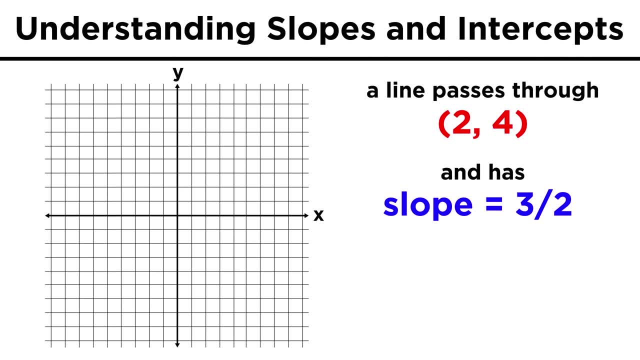 We could say that a line passes through two-four and has a slope. We could say that a line passes through two-four and has a slope. This could be the slope of three halves. To draw this line, we would just go to the point two-four and start applying the slope. 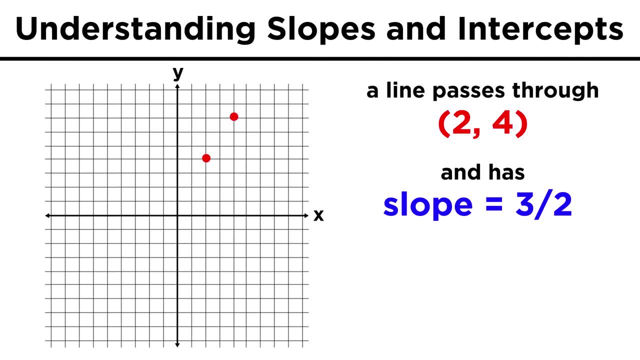 Up: three over two. This could also be down three, two to the left, because negative three over negative two also equals three halves, and that's how the slope, which we can regard as the rate of change, makes sense, regardless of which direction you travel. 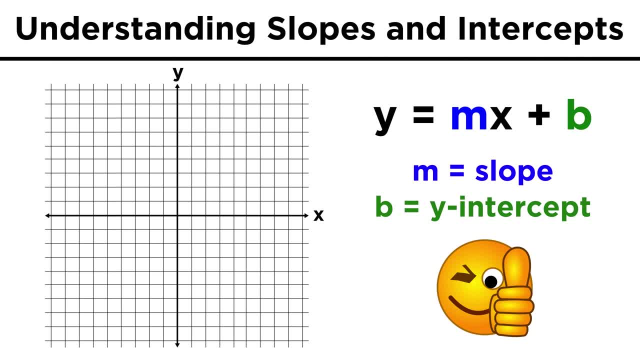 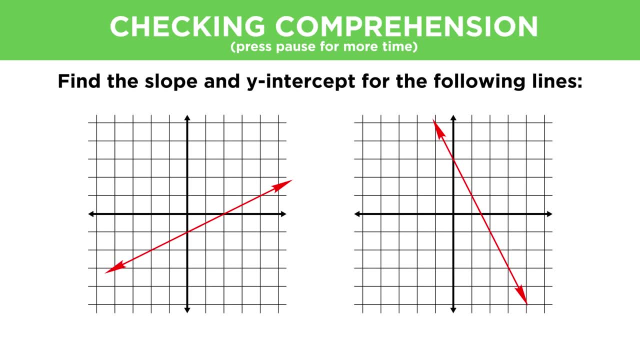 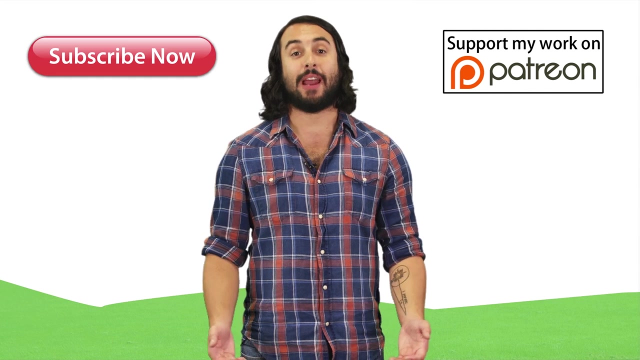 Now that we understand slope and slope, what do we do? I call it the slope and slope. I call it the slope and slope and Y-intercepts. Let's check comprehension. Thanks for watching, guys. Subscribe to my channel for more tutorials. support me on.